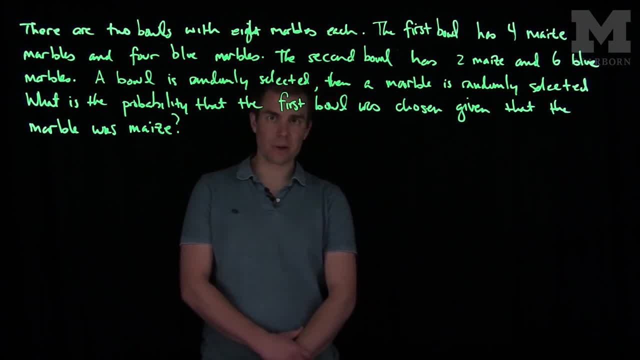 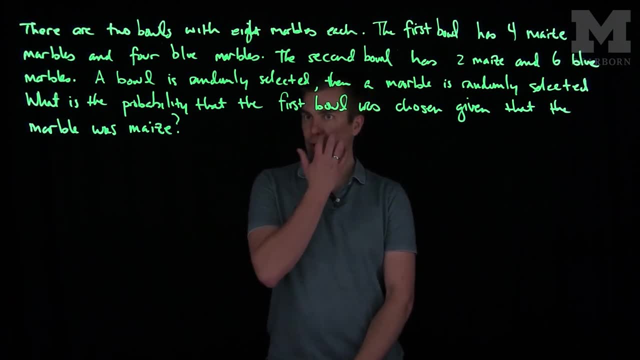 and six blue marbles. A bowl is chosen randomly, and we'll assume that each bowl is equally likely to be chosen, and then a marble is randomly selected from that bowl. We would like to know the probability that the first bowl was chosen, given that the marble was 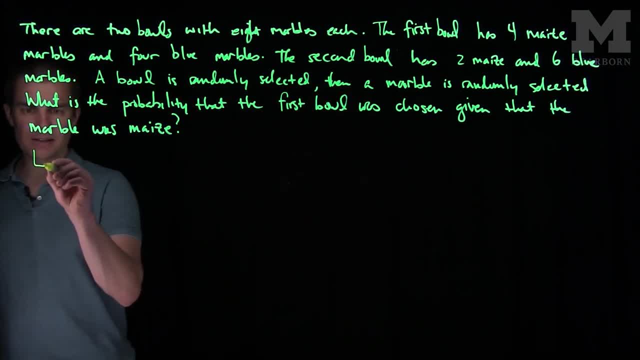 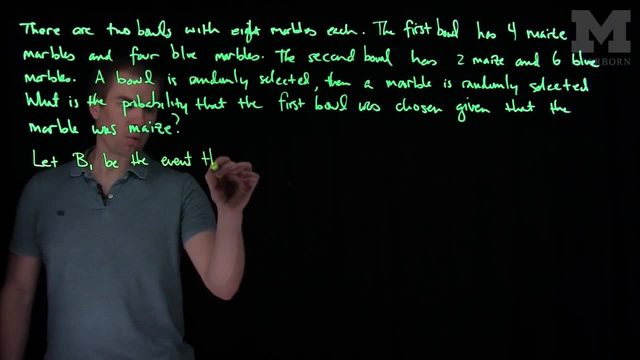 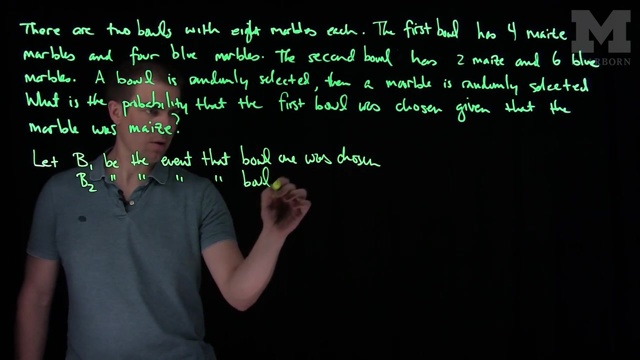 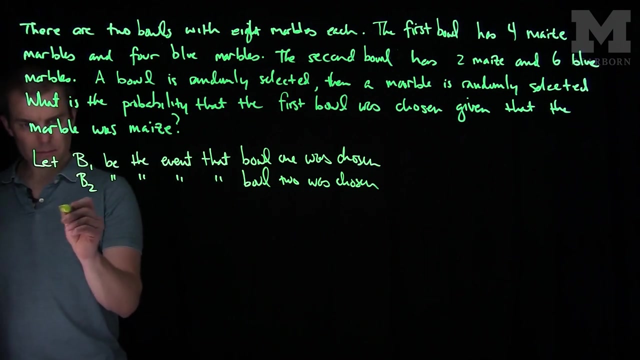 maize. So let's define some events. Let's let B1 be the event that bowl one was chosen and similarly, we'll let B2 be the event that bowl two was chosen. We'll let we have maize. let M be the event that a maize ball, that a maize marble was. 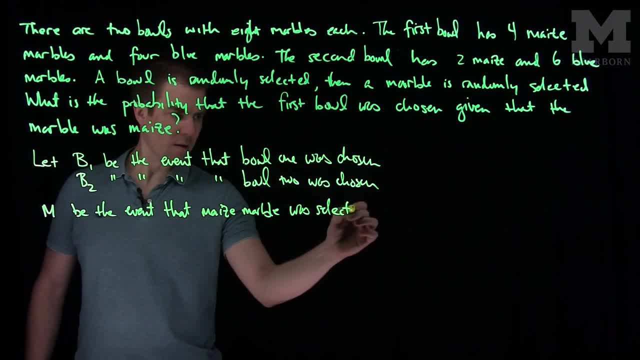 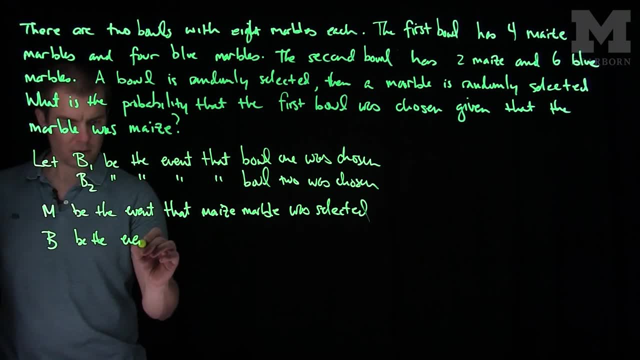 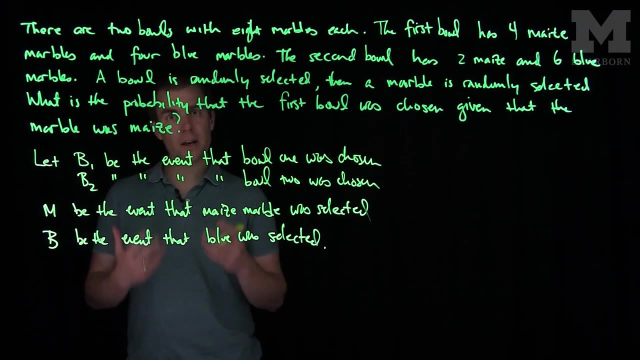 selected, and let's similarly let B, with no subscript, be the event that bowl two was selected, given that a maize ball that blue was selected. It is very important to define these events before you solve the problem We would now. 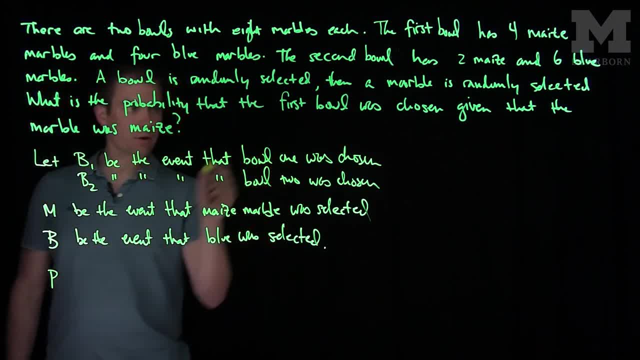 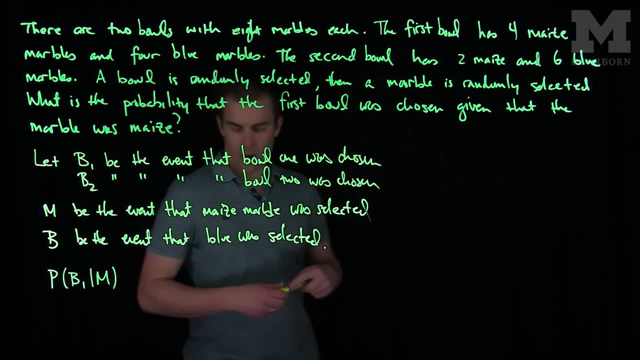 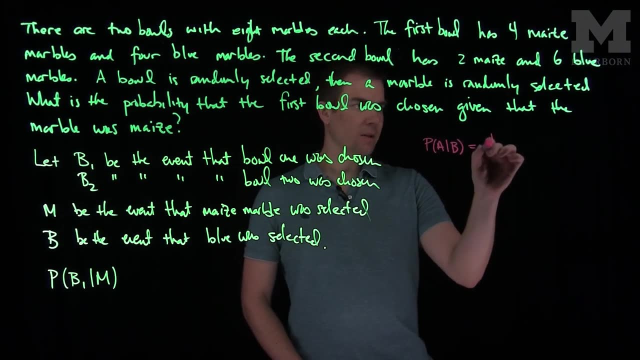 like to find the probability that the first bowl was selected- B1, given that maize was selected. Now we recall the definition of conditional probabilities. We recall the probability of A given B. is the probability of A and B over the probability of B? 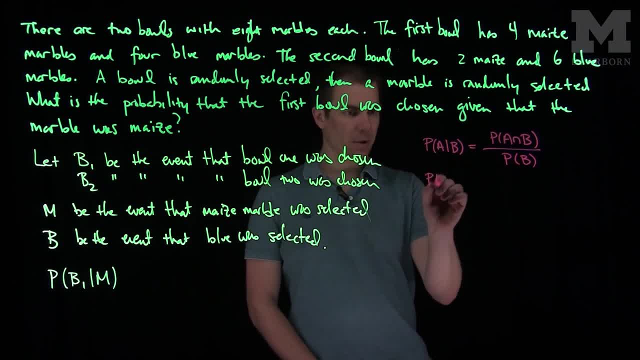 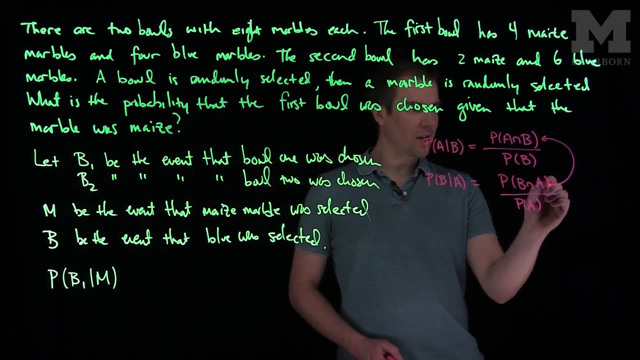 We can use this relationship in the reverse order and say the probability of B given A is the probability of B and A over the probability of A. So we can notice now that both of these two expressions on the numerators are the same. These are equal. 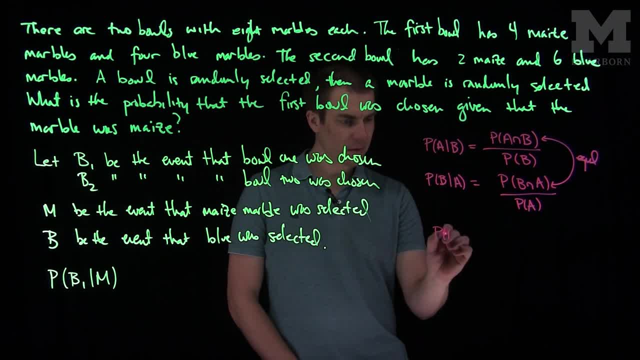 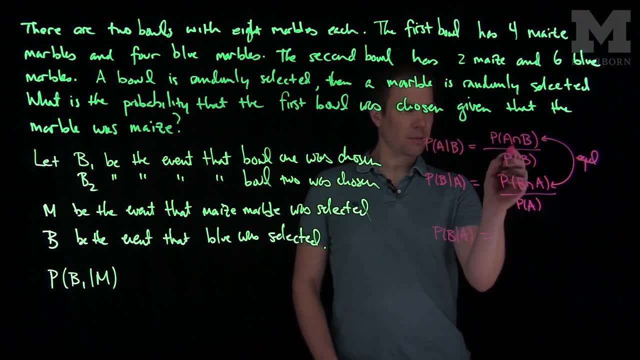 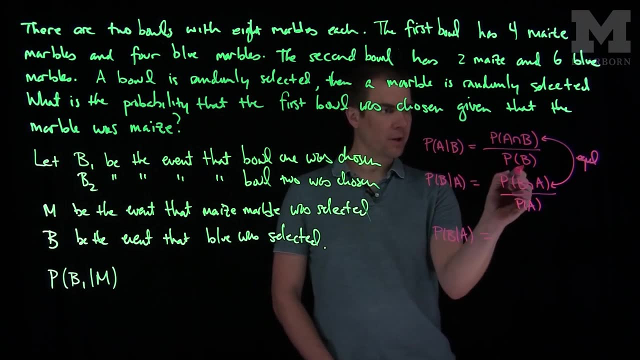 And so what we can do now is we can replace the probability of B given A with Well, the probability of B given A is this: probability A and B, which we can write as the probability. So this on top over here will be the probability of B. 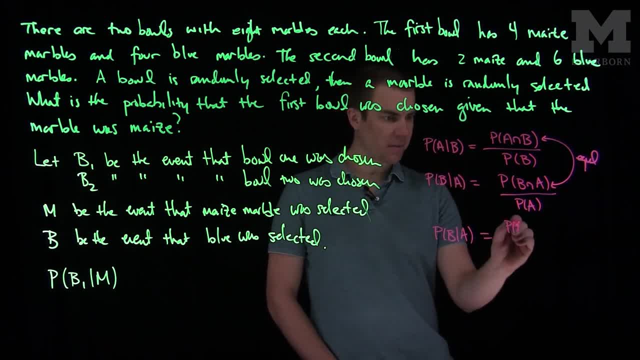 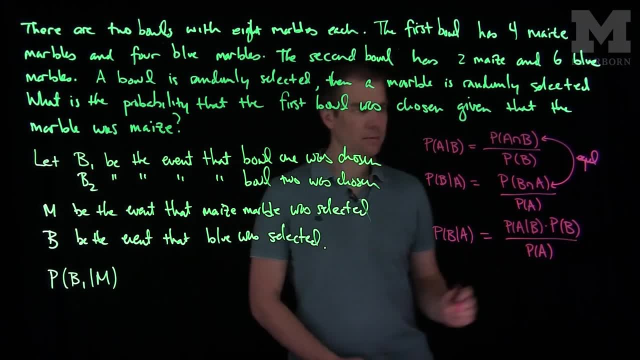 times the probability of A given B. So I'll have the probability of A given B So I can flip the order Times the probability of B divided by the probability of A. So we'll use this relationship. This is a form of Bayes' theorem.